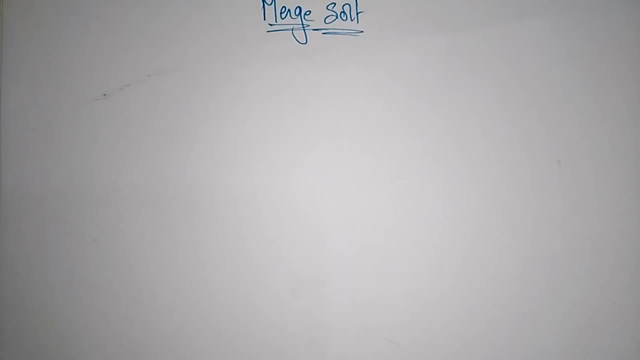 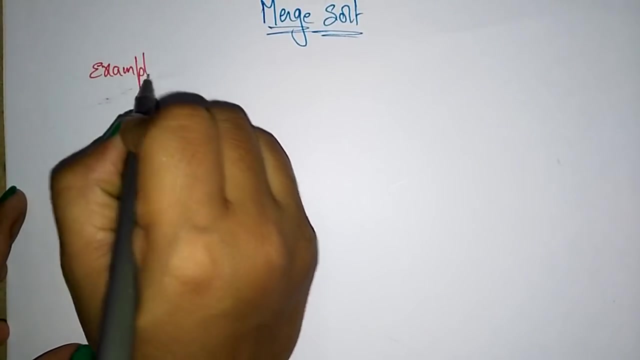 Students. in the previous video I explained about what is a merge sort and algorithm of the merge sort. Now let us see the example for the merge sort. So let me take one array. Let's see the example how we merge an array. 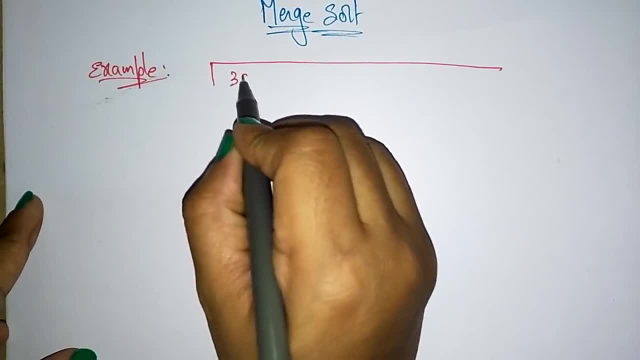 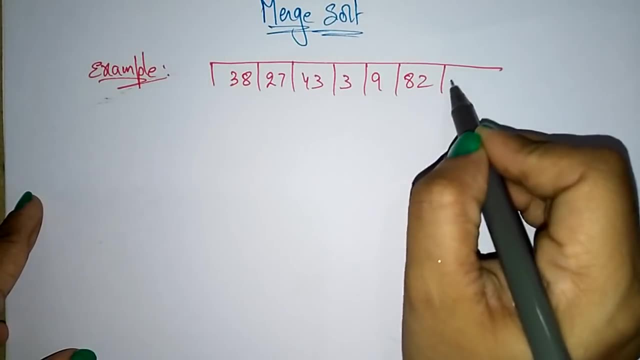 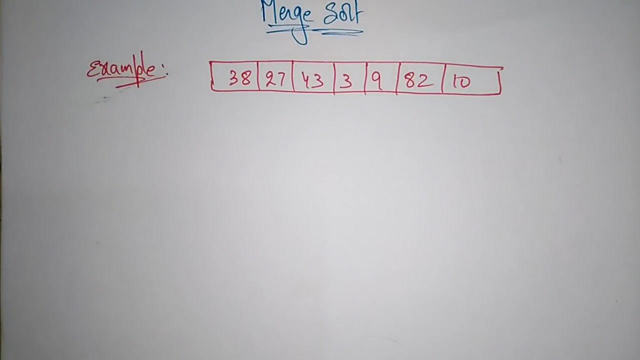 38,, 27,, 43,, 3,, 9,, 82 and 10.. So this is an unsorted array. We have to sort this array by using merge sort technique. So what is the merge sort technique? First you have to divide, just like divide and conquer. So this is an example of divide and conquer method. So divide and after that you have to. 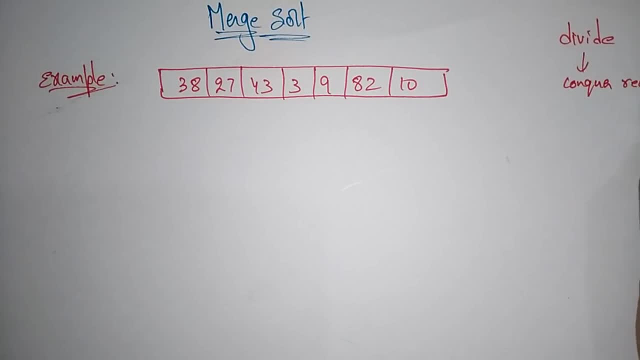 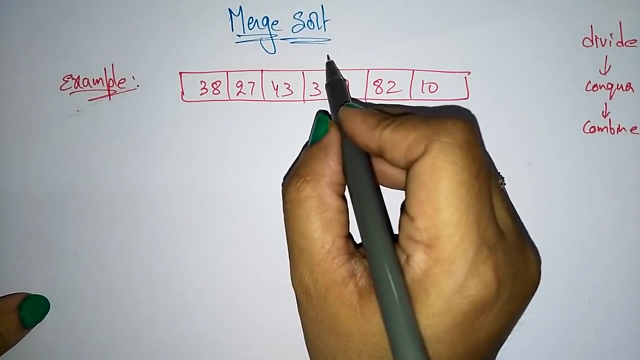 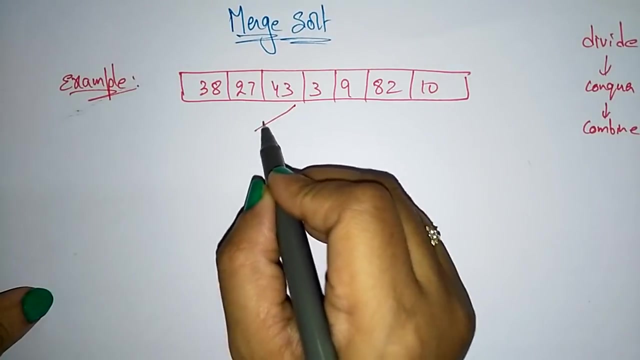 conquer recursively. So after that you have to combine. Combine means merge. So now let us see. So this is an array. Now I am dividing this array into two halves. So this is the size of n. Now I am dividing this size of n into two halves, n by 2.. So in the first half I am having the elements like 38,. 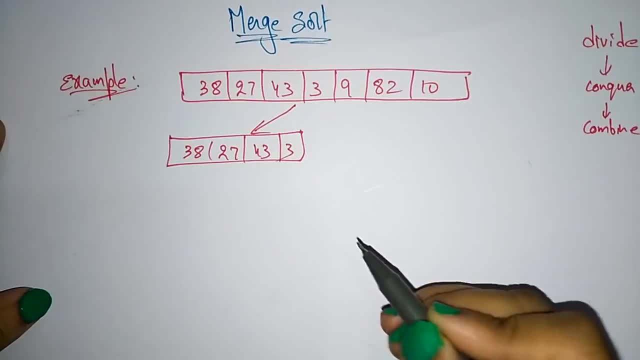 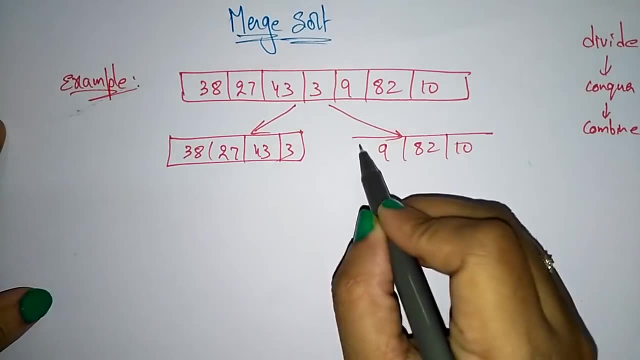 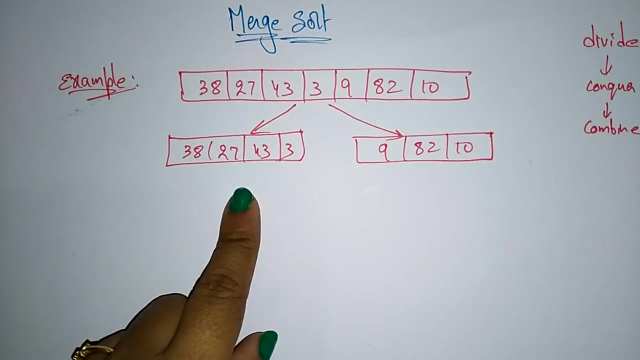 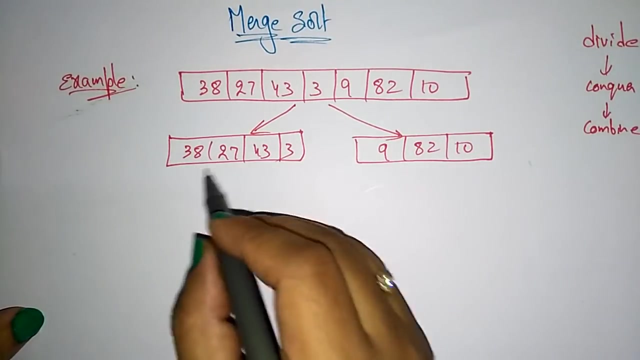 27,, 43, 3 and another half 9,, 82,, 10.. Okay, So now I divide this array into two halves. So after that again I am dividing recursively, After that I will sort Now divide this array into two halves. 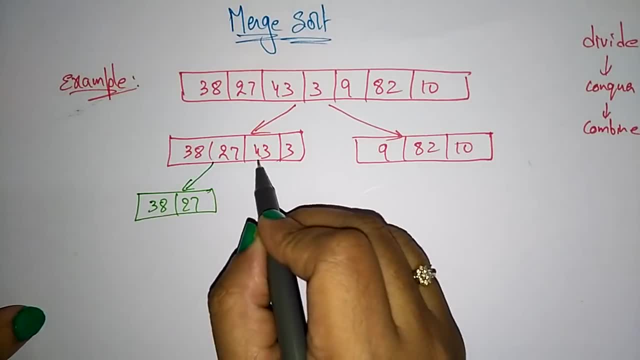 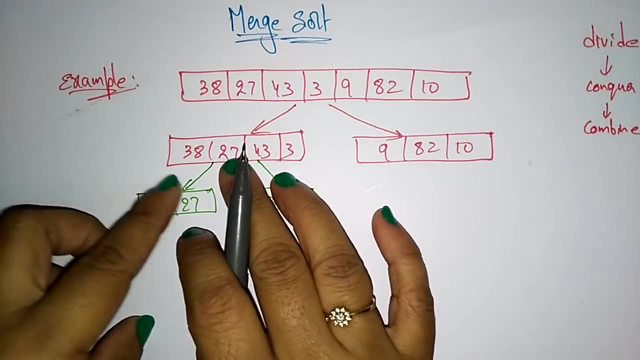 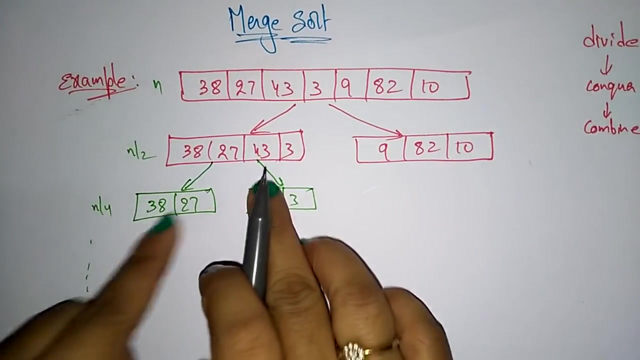 38, 27.. Again, this 43 into 3. So this array of size n by 2. This is n, n by 2. Now n by 4. Like that. So I divided this array again into two halves. So in the same way here also. 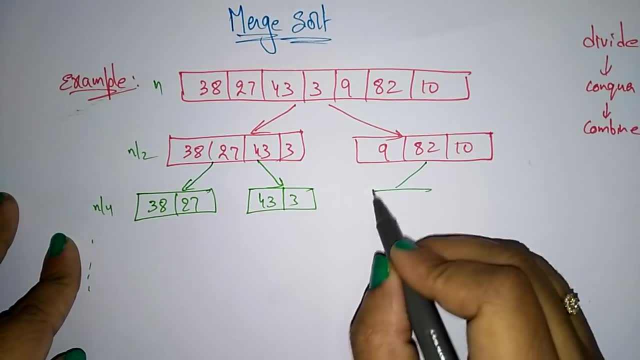 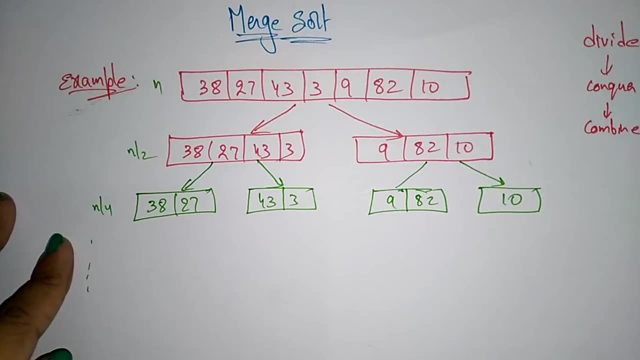 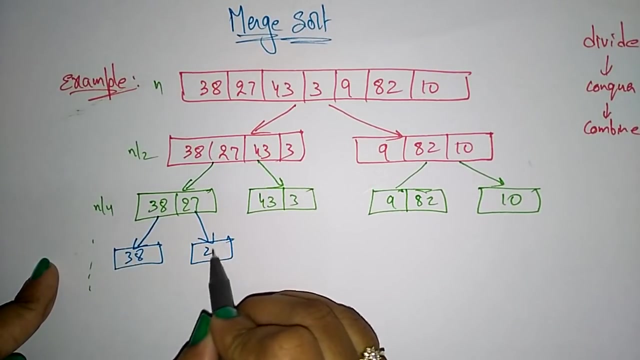 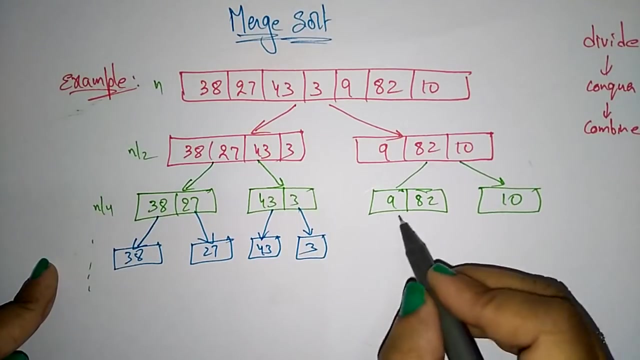 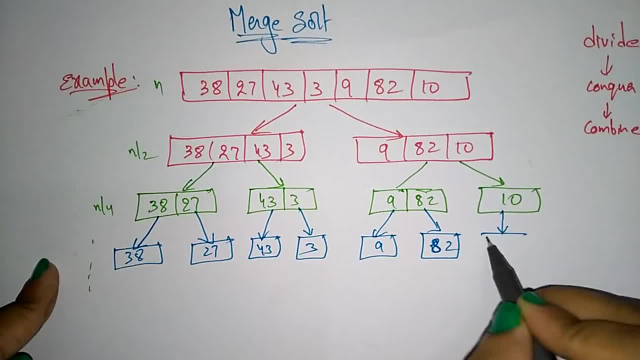 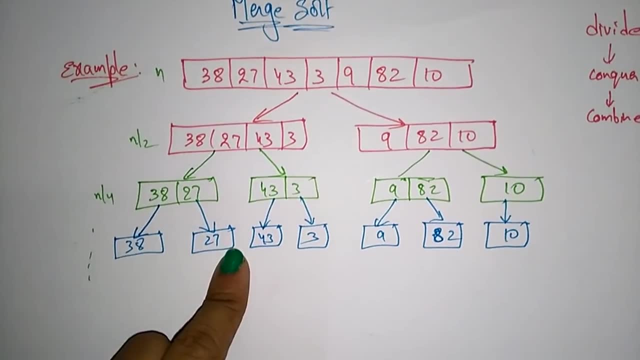 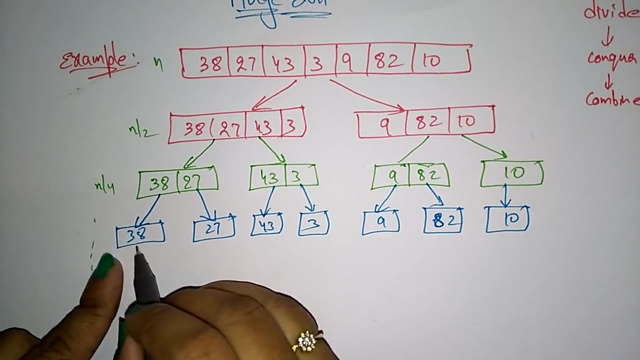 and 10. so this is conquer recursively is over, means all elements are come to one. but the size of one, the array size, is one. now combine the array by sorting, just combine these two array by sorting. so 20, 38, 27. which one is the smallest one? 27, 38. 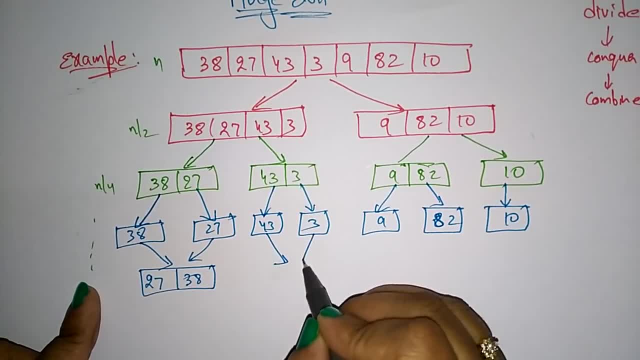 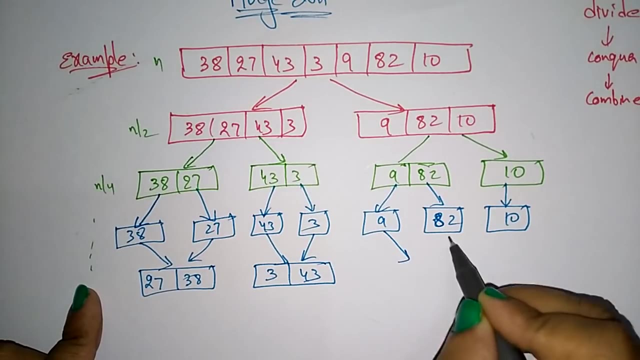 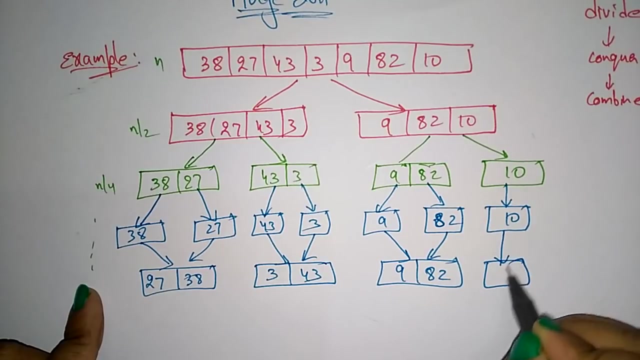 okay, you have to combine the array by solving the problem. that is a merge sort. so combine the array by solving the problem. so just sort this 343. so here also, you just sort this 9, 82 and 10. so this is a technique, technique of merging. so here i am merging the array. 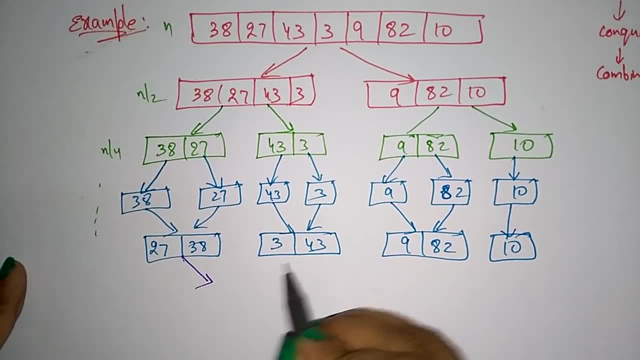 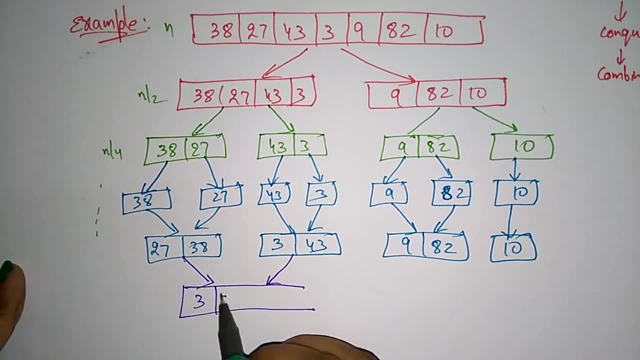 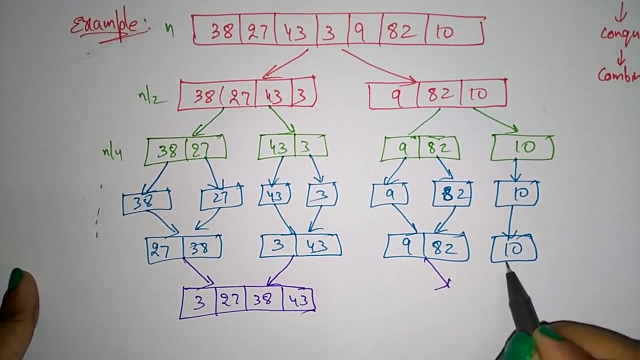 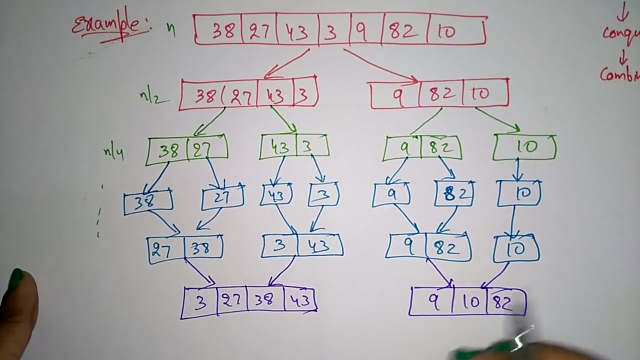 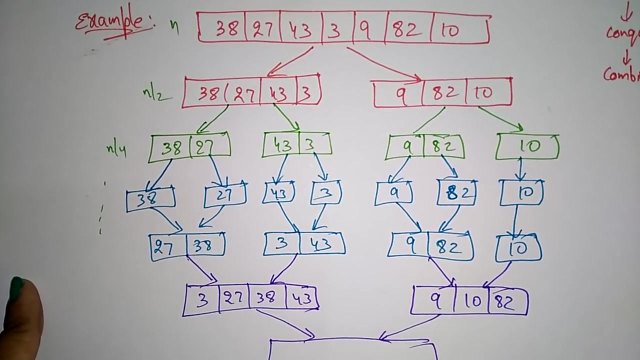 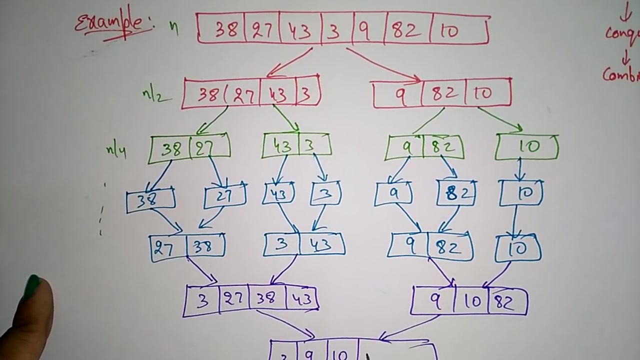 so again now i merge these two arrays by solving the problem three. so in this: 27, 38, 43. okay, again merge these two arrays sub, sub arrays. you call it as sub arrays: 9, 10, 82. okay, again merge these two arrays by sorting. so in this, least one is three, after that 9, after that 10, after that 27, next 38, next 43.